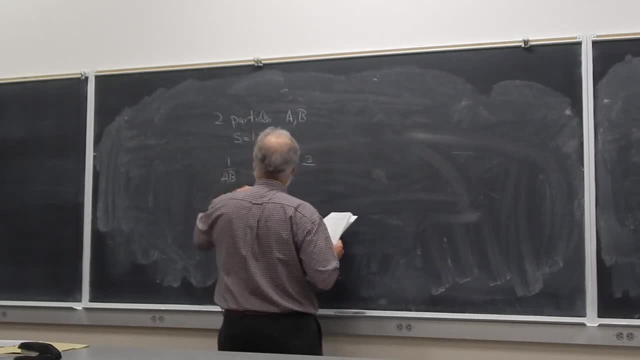 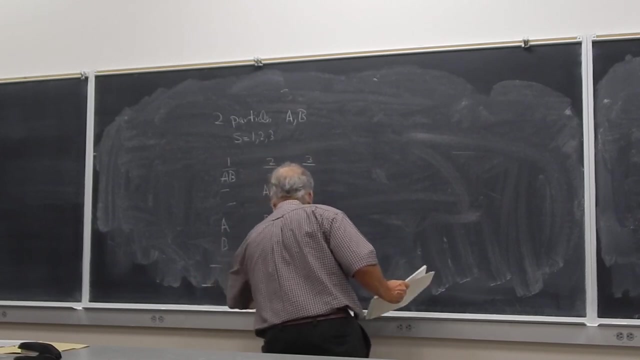 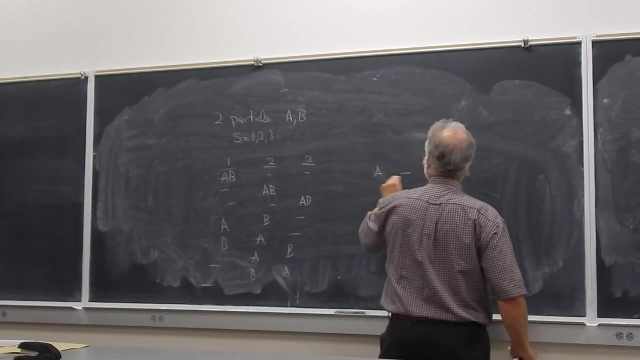 So the possibilities are fairly large. I can have one, I can have both particles in each of the three states, and I can have a situation where I have one particle in two of the three states And then we're running out of room over here. so now we can have A slash B and B slash A. 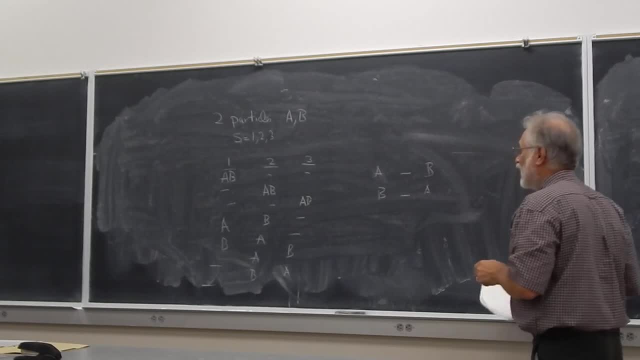 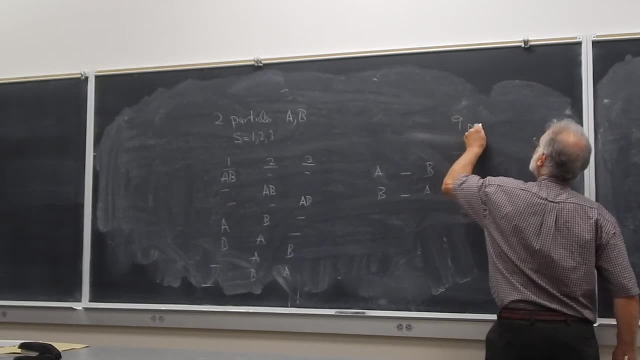 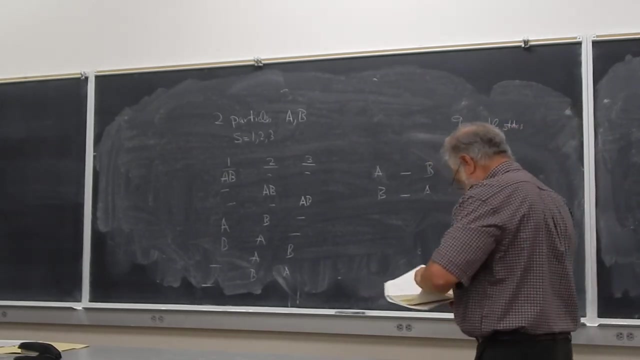 And that gives us a total, should give us a total of nine states, doesn't it? One, two, three, four, five, six, seven, eight, nine possible states in classical statistics. So let's move to the quantum statistics. 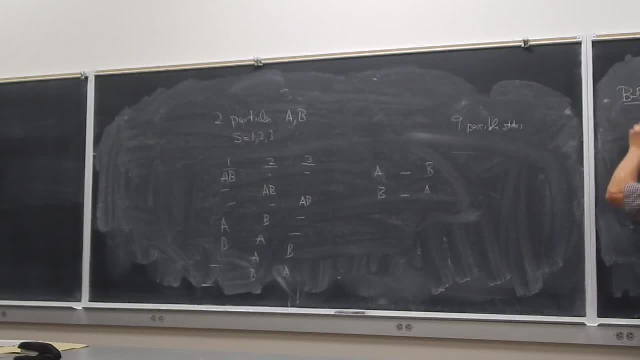 So suppose I were looking at Bose-Einstein statistics. Bose-Einstein statistics, I have one, One, two, three states, But particle A and particle B are indistinguishable from one another, so we might as well just call them both particle A. 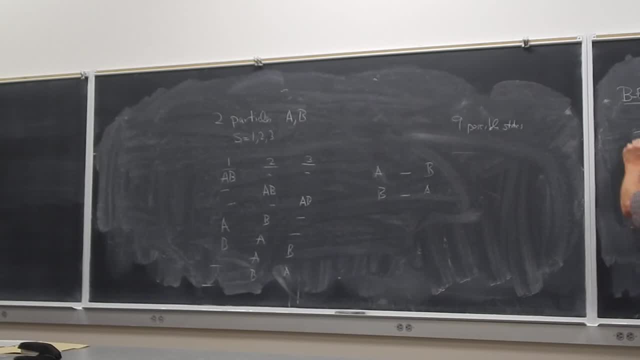 That being the case, because I have no limit on the population of the states, I could have them both in state one, I could have them both in state two, I could have them both in state three, And then they could be distributed one per state. 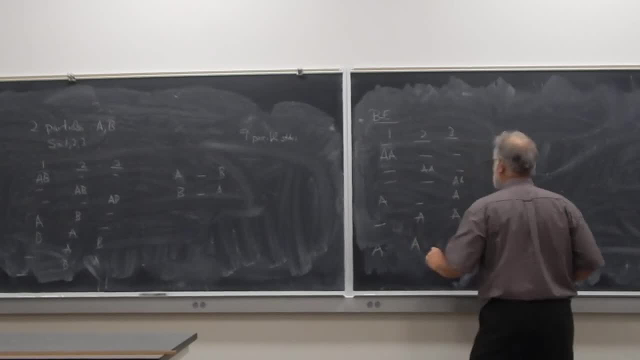 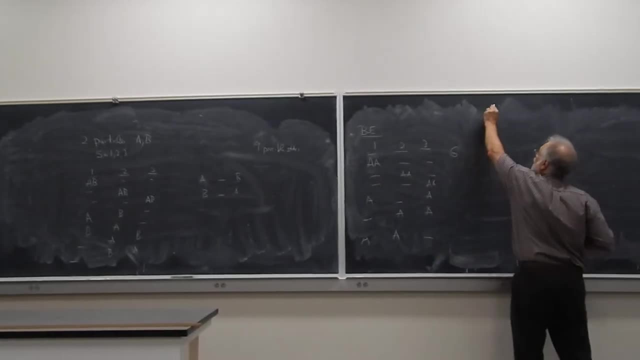 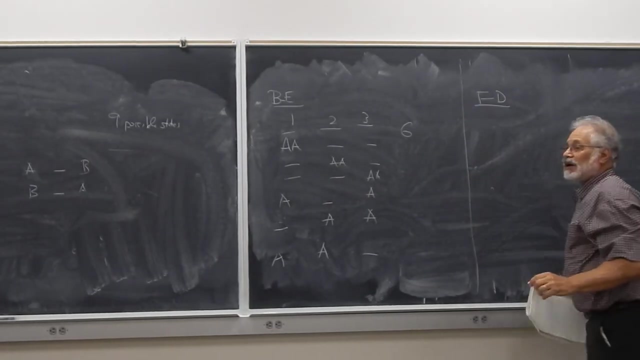 Like so. So in this case, I have six possibilities. Thirdly, let's talk about Fermi-Dirac statistics. Fermi-Dirac statistics: the particles are also indistinguishable. I'll just refer to them as particles A. 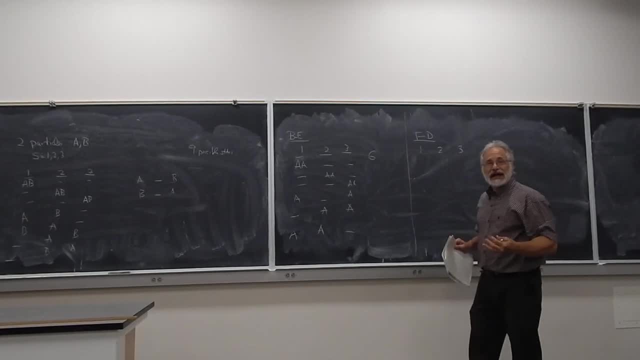 However, there's a limit of one particle per state when I use Fermi-Dirac statistics. Therefore, the only way to do that is to use Fermi-Dirac statistics. Therefore, the only way to do that is to use Fermi-Dirac statistics. 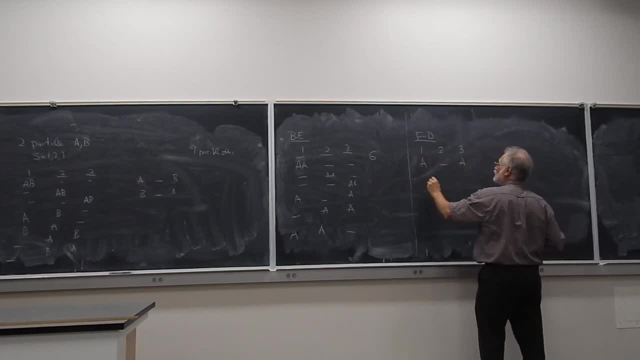 Therefore, the only way to do that is to use Fermi-Dirac statistics. If I only have three possibilities, they can either be in states one and three, they can be in states one and two, or they can be in states two and three. 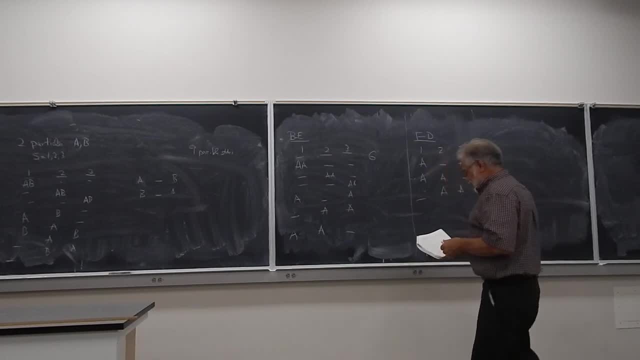 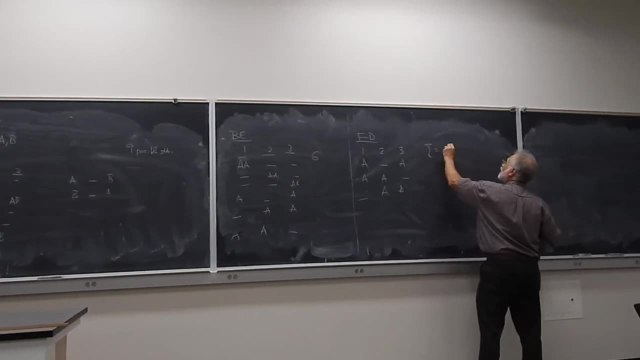 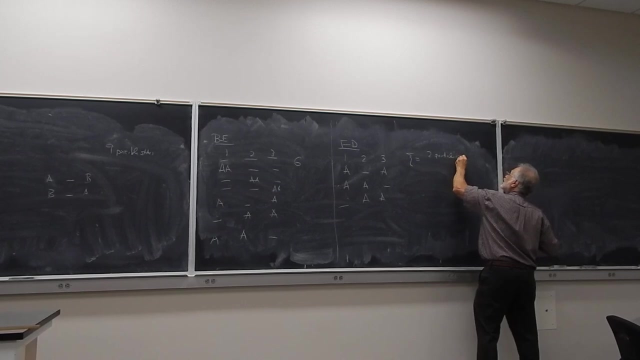 That's it. Those are the only choices you have For further examination. let's define the quantity eta. I'm sorry C C to be the probability that two particles are in the same state divided by the number of particles in between. 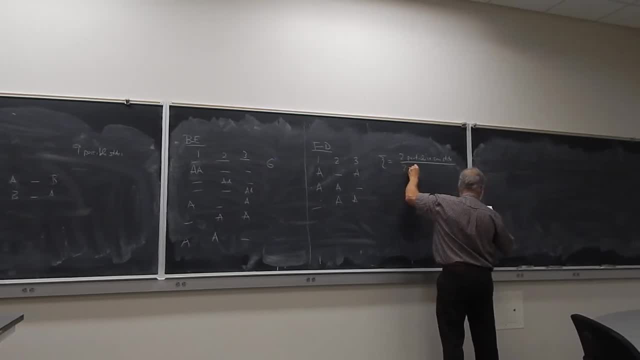 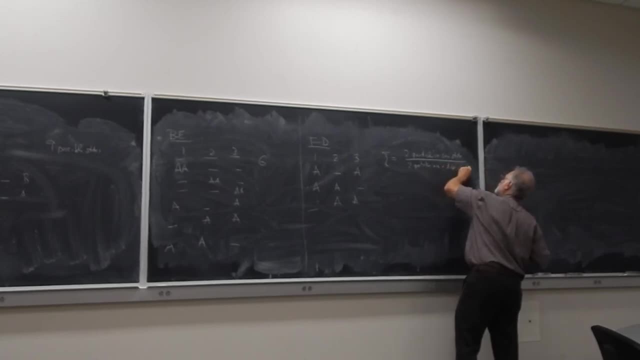 by the probability that two particles are in different states, and so, in the case of Maxwell Boltzmann, C turns out to be three out of six or one half. in the case of Bose-Einstein, we have a three out of three or one, and, of course, in 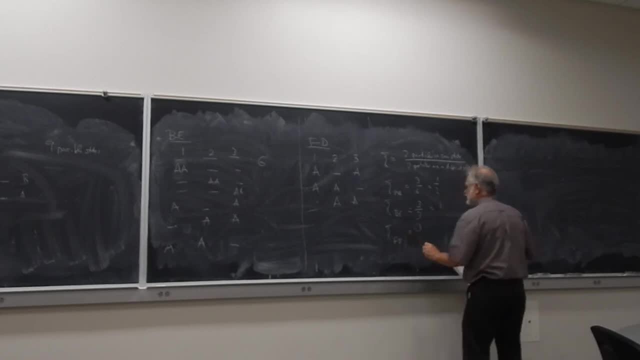 Fermi-Dirac, none of them can be in the same state, and so that's just going to be zero. so what that says is that the particles tend to bunch together more in Bose-Einstein statistics than classical statistics, but they are farther apart in Fermi-Dirac statistics as compared with classical. 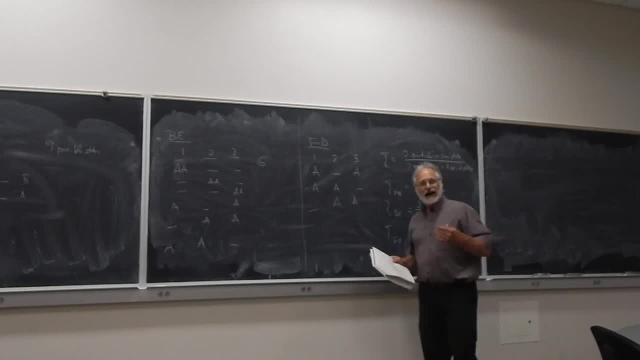 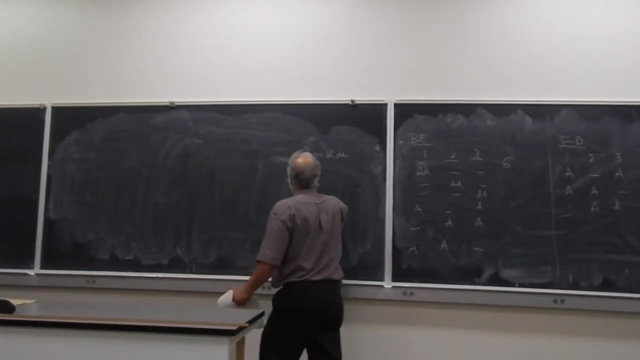 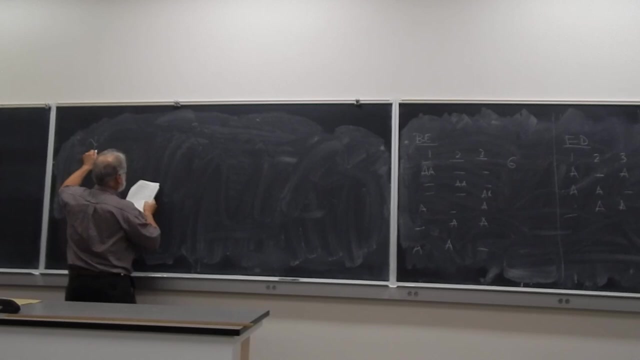 statistics. Okay, so that's a really simple illustration of how we can compare the two quantum distributions to the classical statistics. let's do it. let's do this in a little more sophisticated way. let's look at, very briefly, the wave function might look like. so let's say, little psi sub S of Q is a one. 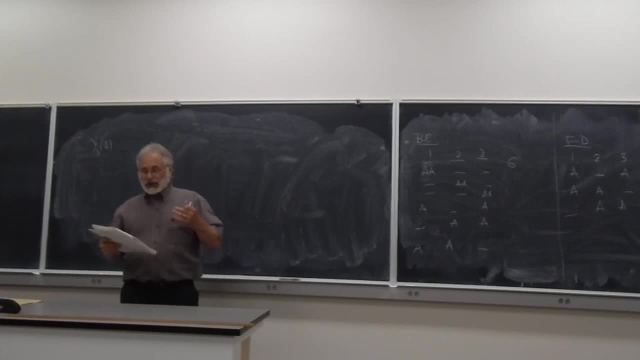 particle wave function for a single positive factor, which is one particle. single particle with coordinate Q in state S. okay, And then let's talk about capital psi being the state for the entire gas. So it's a wave function for the entire gas, and 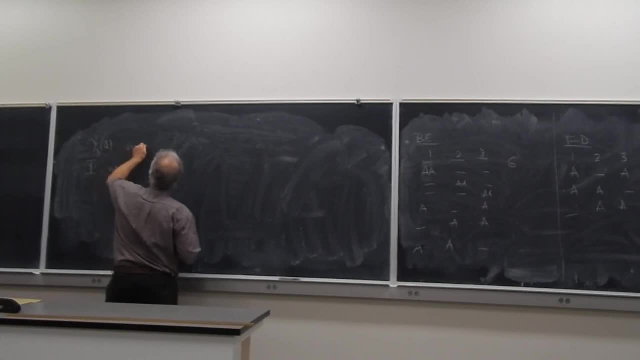 psi is a one-particle function. okay, Since the particles are not interacting, let's write capital psi as just a product of all the one-particle wave functions. That's simple enough. Now let's look at what the three statistics, how they would view the wave function. So 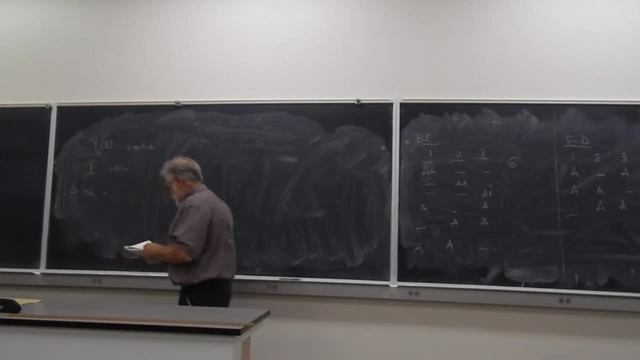 first of all, let's look at Maxwell-Holtzmann statistics. You have no symmetry requirement on psi. If I exchange particles. that is going to be an issue with Bose-Einstein and Fermi-Durant, as we stated last time. So a complete set of wave functions, capital psi would be the. 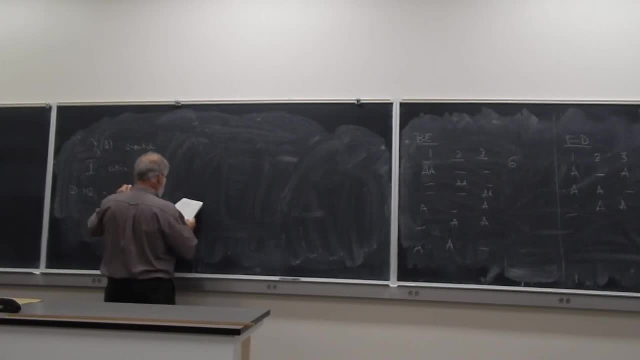 nine functions that look like psi. So I of QA, psi sub J of QB, And now we get nine functions multiplied together. In Bose-Einstein statistics we have a symmetry requirement. It says that psi must be capital, psi must be symmetric under particle exchange. 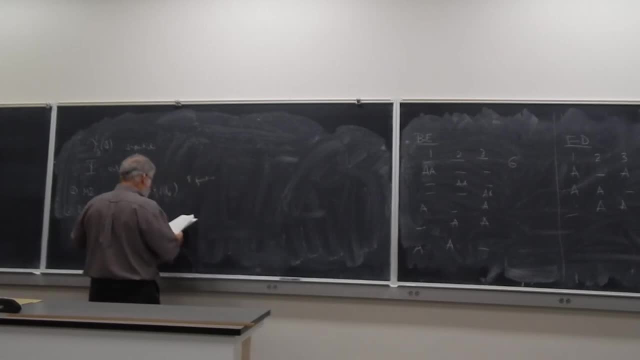 So what has to happen there is I can write. then I'm going to get three wave functions that look like psi sub I of Q of A times psi sub I of Q of B, because they're the same particle in both states, for I equal 1,, 2, and 3.. I will also get three functions of 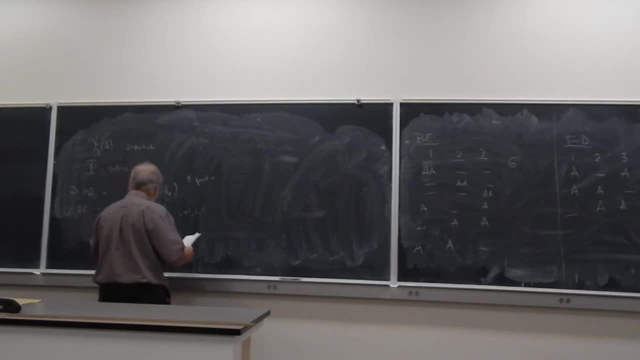 the form psi sub I of QA times psi sub J of QB. So I can write: then I'm going to get the same function of psi sub J of QB times psi sub I of QB times psi sub J of QB, plus psi sub I of QB plus psi sub J of QA, So that's a symmetric wave function and Bose-Einstein. 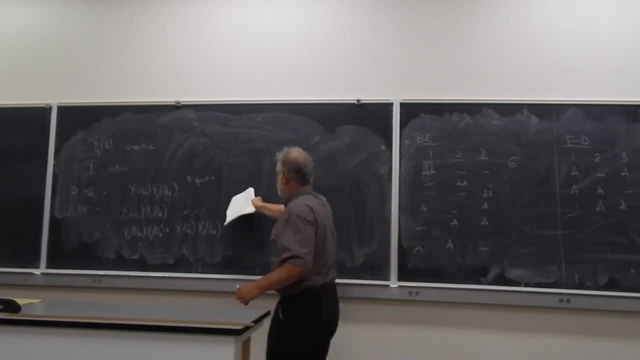 requires symmetric wave functions. So I've got three here and I've got three from here. These three, of course, are when they're in the same state. These three are when they're in different states. Finally, in the Fermi-Dirac case, it's quite simple. 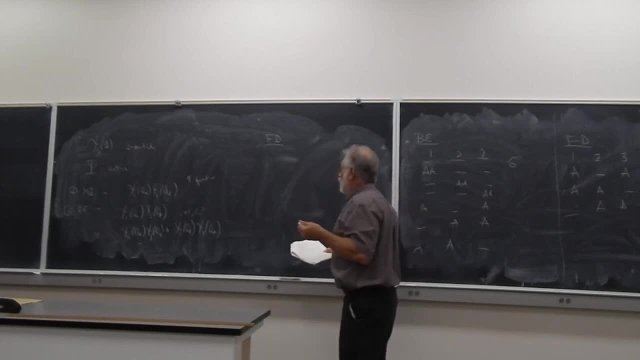 Psi, capital. Psi must be anti-symmetric. Well, when I exchange two particles, therefore, I have something that looks like this: I have Psi i of qA, Psi j of qB, minus Psi i of qB, Psi j of qA. 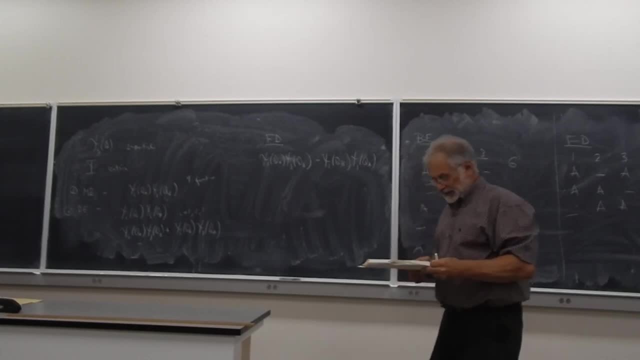 So this illustrates the symmetry and anti-symmetry of the wave functions for each of those three cases. That's a nice representation, but it's probably more interesting to see: okay, how do these guys work? How do these statistics work? 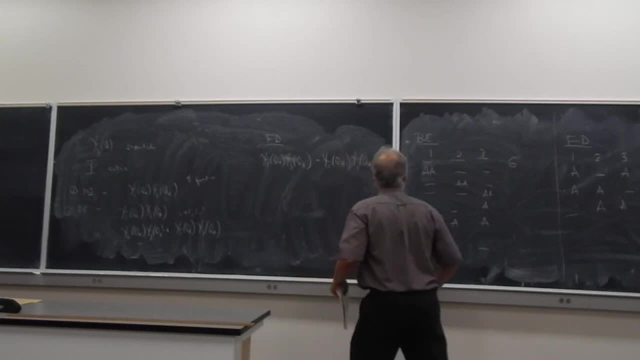 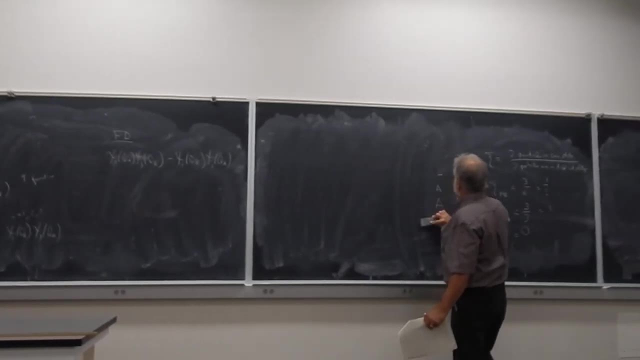 So I'm going to formulate right now a statistical problem And we're going to essentially solve- We're going to solve it with all three distribution systems And then we'll go deeper and deeper into the systems themselves. So here's the statistical problem. 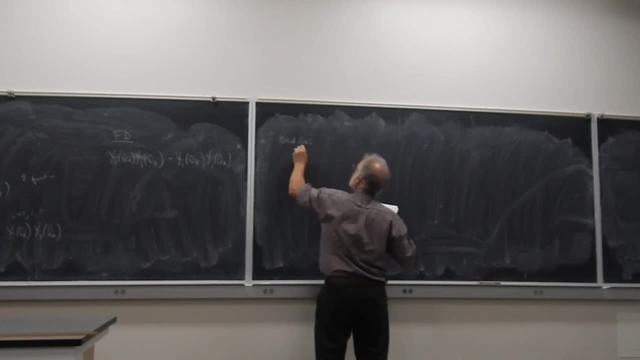 I have an idea: gas in a container. The container has a volume, V. It's an equilibrium at some temperature, T, The possible quantum states of a single particle could be R, could be S, could be any letter, I like it. I like the energy of a particle that's in state R would be V sub R. 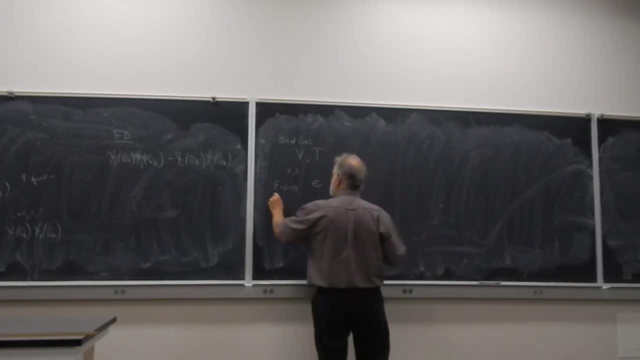 And for S it would be V sub S, The number of particles in state R. I'm going to call that N sub R And I'm going to talk about the possible quantum states in the entire gas. So for the entire gas I have some. 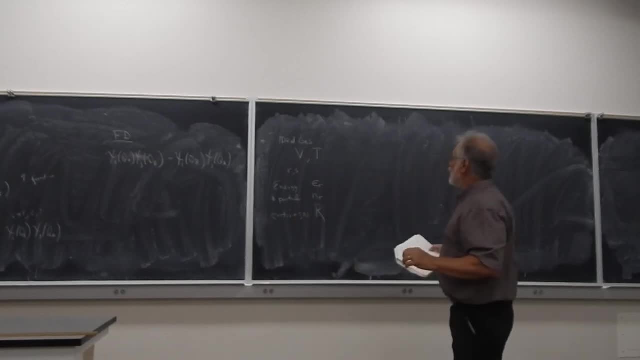 I have some R number of quantum states. The total energy I would expect for that gas would be just the sum of all of the energies of the individual states and particles in those states, And so I can write that as sum over R, N, sub R, V, sub R, summing up all accessible states. 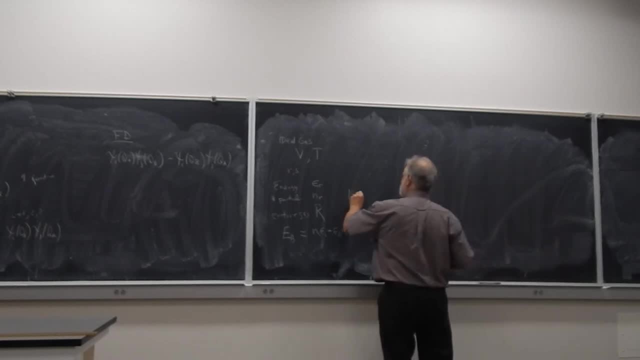 And, of course, the total number of particles. by the same token, I would expect would be the sum of all the particles in each state. Not a big surprise here. Moreover, because it's going to be very interesting to me, I want to know how can I write the partition function. 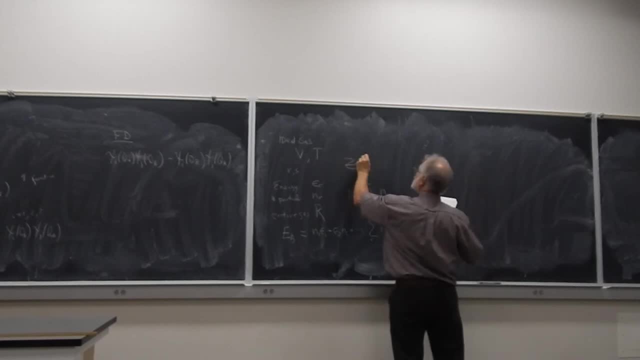 The partition function for the whole gas. I can write as sum over capital R E to the minus beta E sub R, which I can write as the sum over R E to the minus beta N sub 1, epsilon 1, N sub 2, epsilon 2,, all the way up to however many I have in the gas in these states. 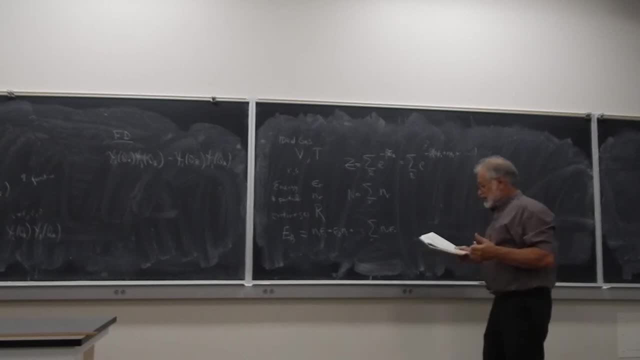 Now suppose I have a given state. Suppose I want to call S the state that I'm interested in, If I want to find the mean number. Again, this is not anything new compared to what we've been doing, But suppose I want to find the mean number of states in state S. 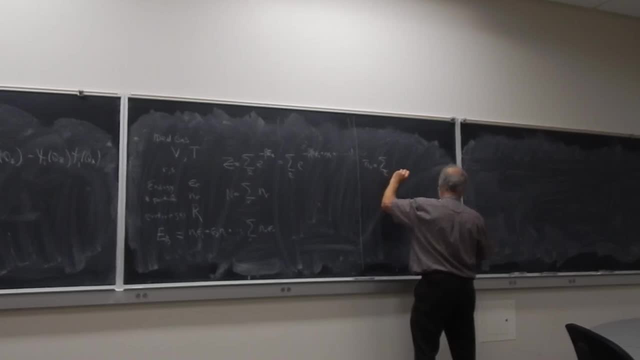 Mean number of particles in state S. I'm sorry, That's just going to be the sum over R, N, sub S, E to the minus beta: N1, epsilon 1, N2, epsilon 2,, all the way up. 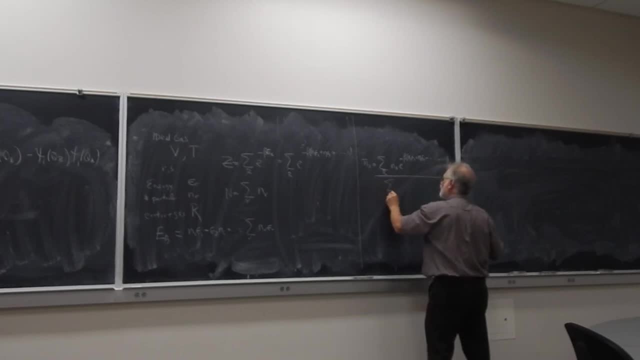 All divided by, of course, sum over R, E to the minus Beta N1,, epsilon 1, plus all the way up. Okay, Or that divided by Z. if you will, Then for a again, I can write this as minus 1 over beta times. Z divided by sorry times, the partial of Z with respect to the energy. 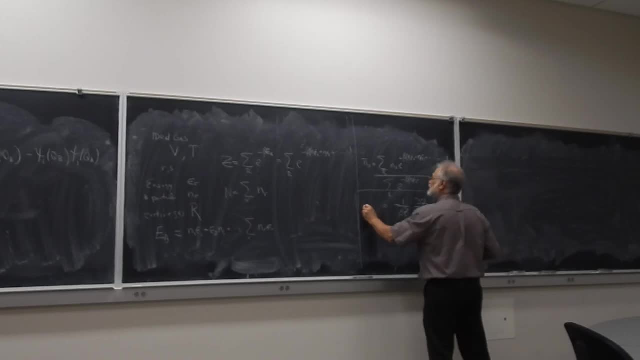 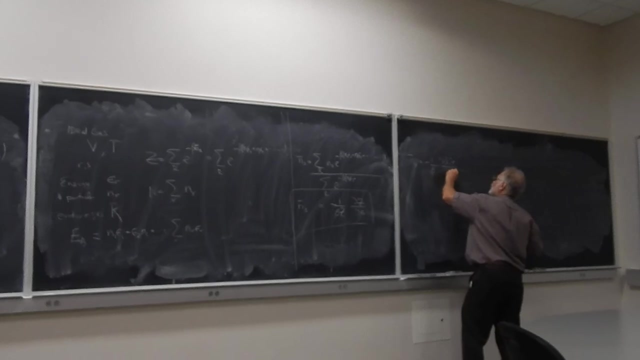 Okay, So that is my mean number of states. I can write that according to the way this is written, This is a logarithmic derivative, as it were. So for any given state, I can write this in a shorthand fashion: Minus 1 over beta times. the derivative of the log of Z with respect to the energy in states. 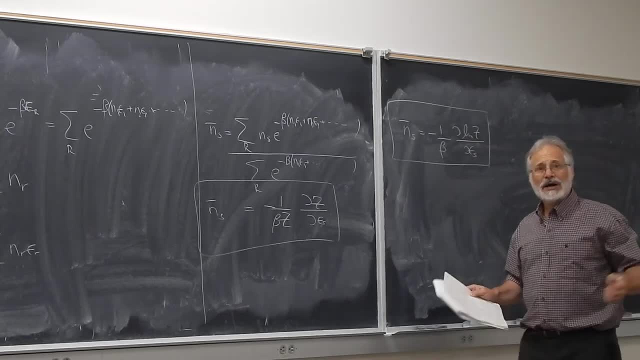 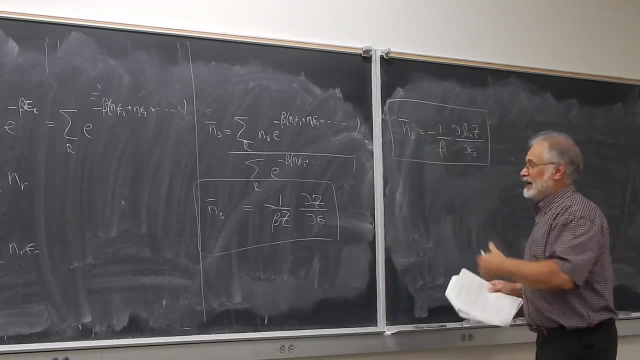 Okay, So that's a nice. That's a nice expression because what we're going to want to do is use these three statistics to come up with mean number of particles in a given state, and also mean energy and possibly entropy and other things as well. 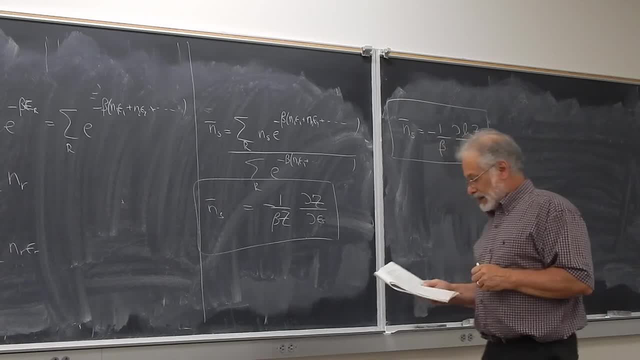 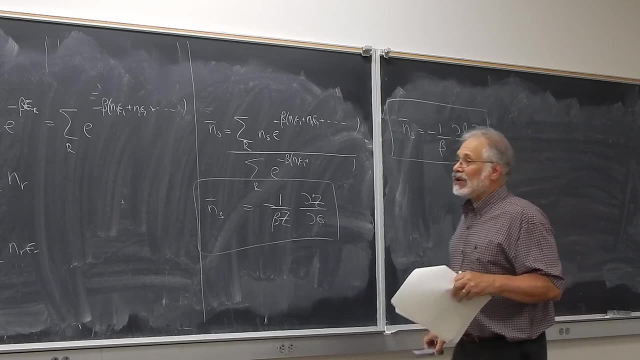 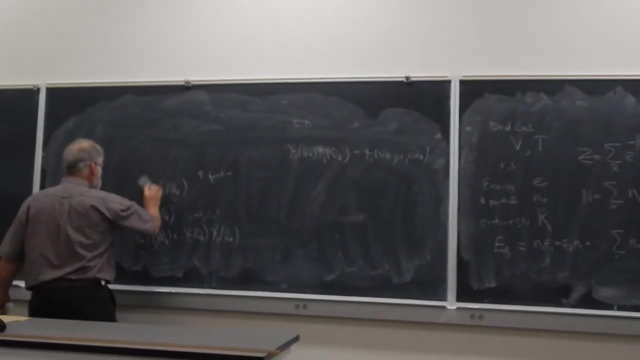 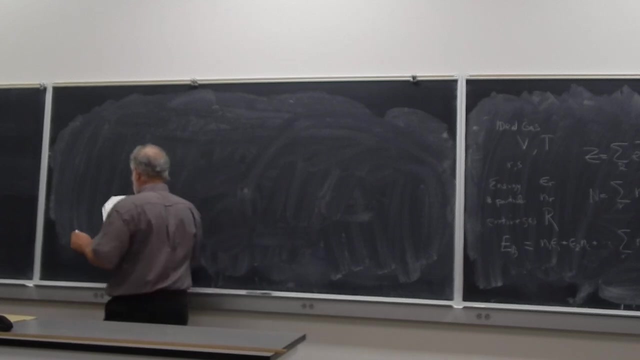 Those are coming down the line. Okay, So this is going to work regardless. Let's see how it works with each of the three distribution systems. So first let's start again with Maxwell-Boltzmann. In the case of Maxwell-Boltzmann statistics, the sum over all particles, all numbers of particles in each state. I can write this: 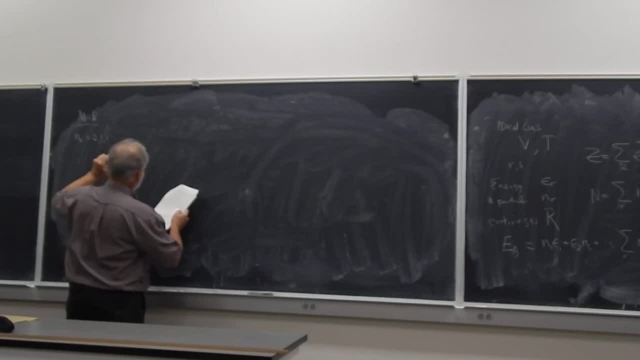 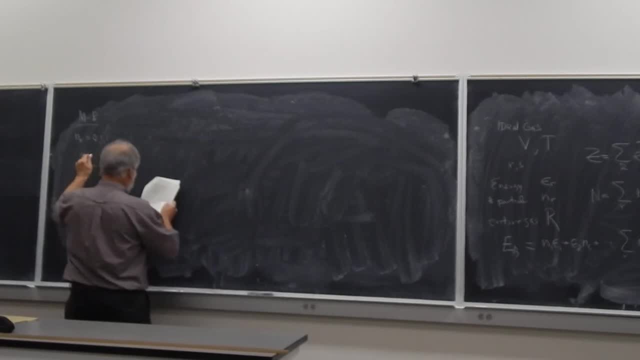 So I can write this as 0,, 1,, 2,, 3, all the way up to whatever number I have for any of the other particles. The only requirement is that if I sum over all those numbers, I'll get the total number of particles in the gas. of course. 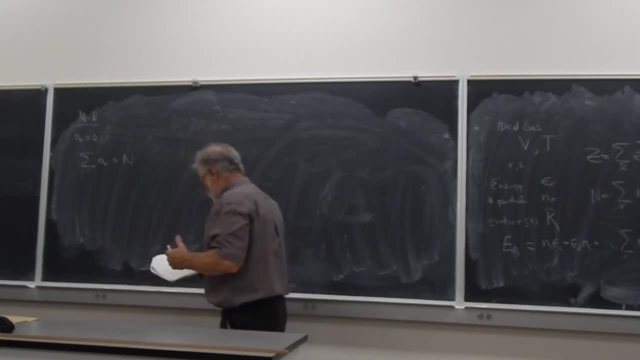 However, these particles are distinguishable, unlike in the quantum cases. So any two permutations of the particles represents a different state, because I can tell one apart from the other. So with Maxwell-Boltzmann, not only do we have to specify how many particles, 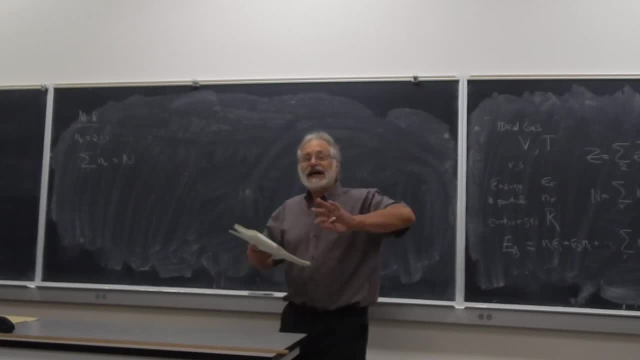 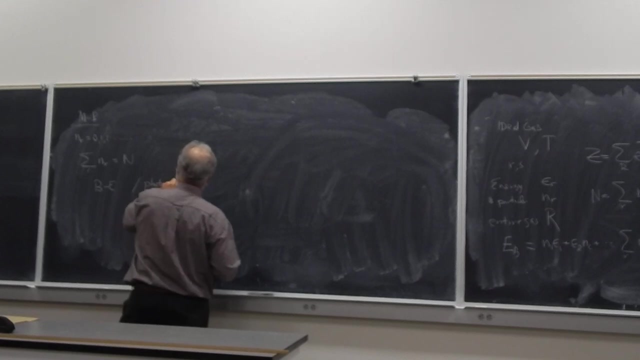 we have to know which ones they are. That's not true for the other distributions. On the other hand, let's look at Bose-Einstein in a more specific way: photon statistics, because photon statistics represents the easiest possible case of Bose-Einstein. 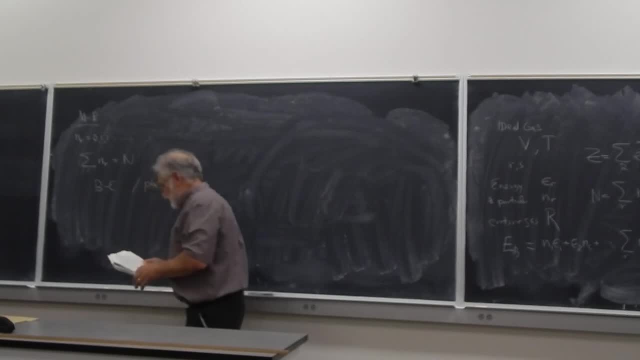 and you'll see that as we go along. Particles are indistinguishable, So all we're concerned with is how many particles are in a particular state, not which ones are which, because we can't tell one from the other. That being the case, I'm interested in something like this: n1, n2, n3, all the way up. 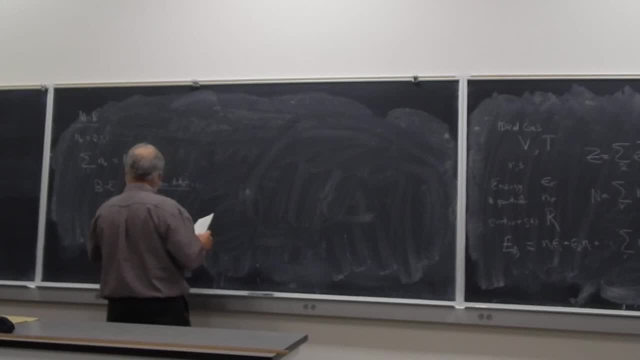 such that I still have a constraint on the number of particles n sub r. but sum over n sub r over r must be equal to the total number of particles. n sub r over r must be equal to the total number of particles. n sub r over r must be equal to the total number of particles in the system. 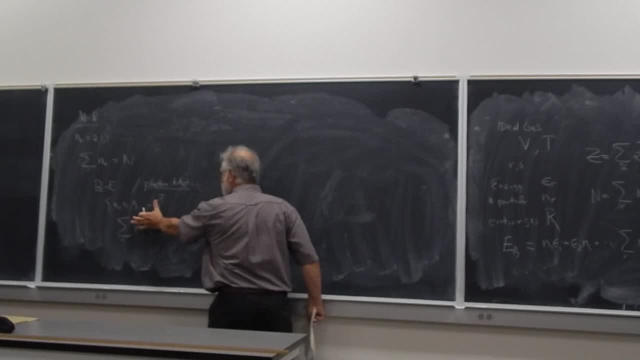 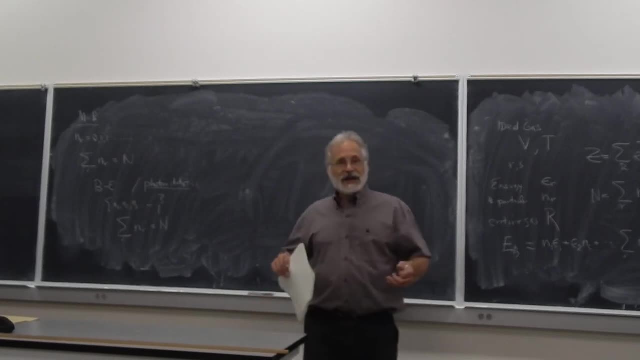 An even simpler case is with photon statistics, where this isn't even a problem. The number of photons that you can create is infinite, and so n is essentially infinity, and we don't have to worry about that constraint, which, as you'll see, will make our lives quite a bit easier. 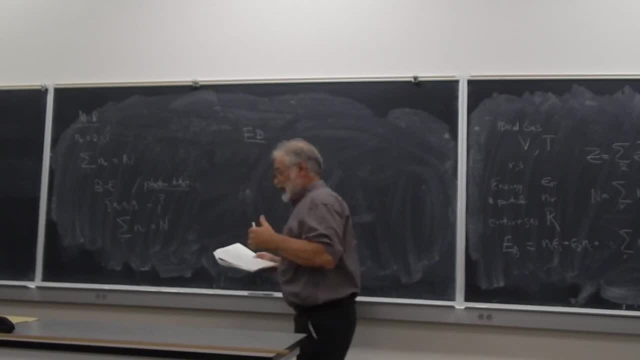 In the case of Fermi-Dirac statistics we still have indistinguishable particles. We can sum over all particle numbers Possible numbers of particles in a state. but in any state the number of particles can be either 0 or 1.. I'm not allowed to have any more than one particle in a state. Remember, that's the way that Fermi-Dirac statistics obey the Pauli exclusion principle. Still have the constraint, though, that the total number of particles will be capital N. 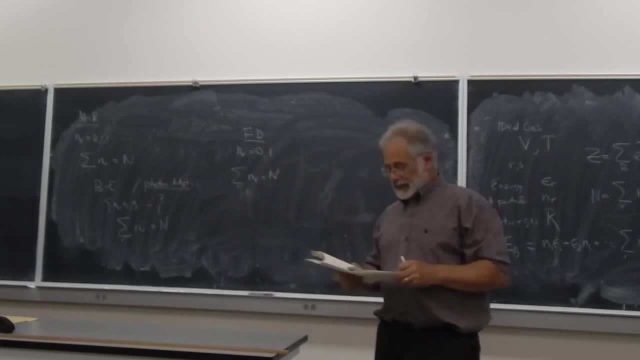 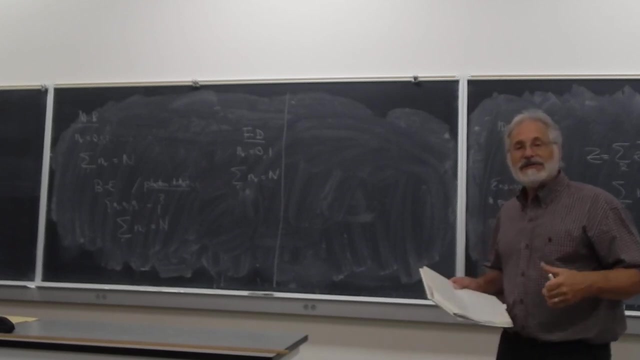 sum over all the particles in all the states. What we want to do now is: let's derive the distribution functions, That is to say, how can we derive, for each of the type of statistics, the mean number of particles in a state? 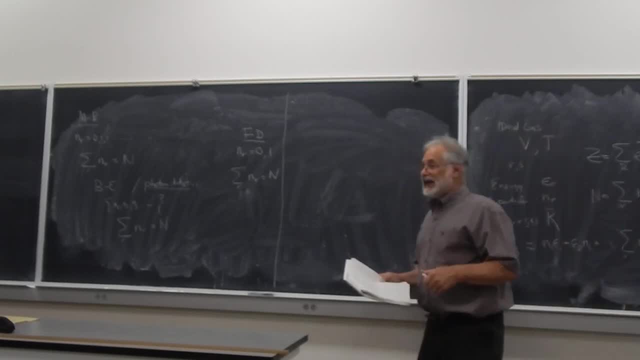 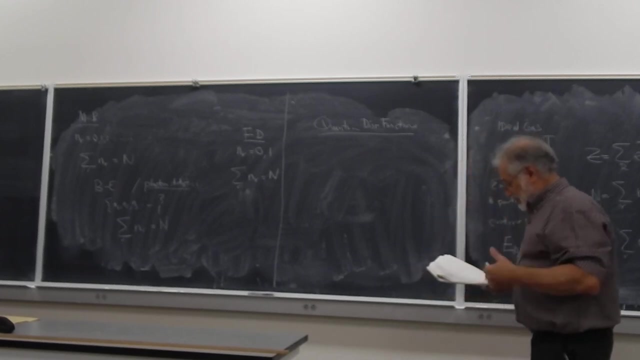 So, first thing we want to say when I'm going to do the quantum distribution functions, The Fermi-Dirac particles are going to be different than particles that obey Bose-Einstein statistics, particularly at low temperatures. By the way, if you go to high enough temperatures, all three statistics will be virtually the same. 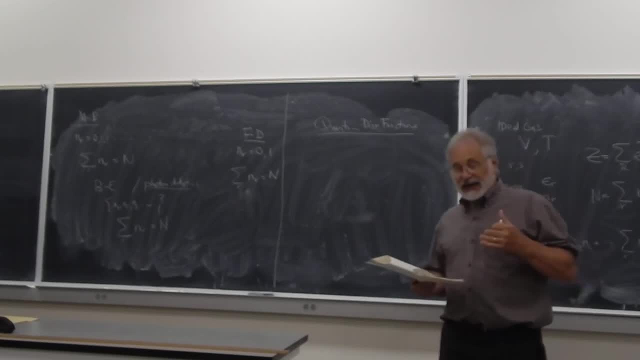 So in this case let's consider a gas of capital, N particles, where the lowest possible energy has some value: E1.. In the case of Bose-Einstein statistics, every single particle in the system could have that energy value. In fact, the lowest possible energy state is when all of those particles have energy, E1.. 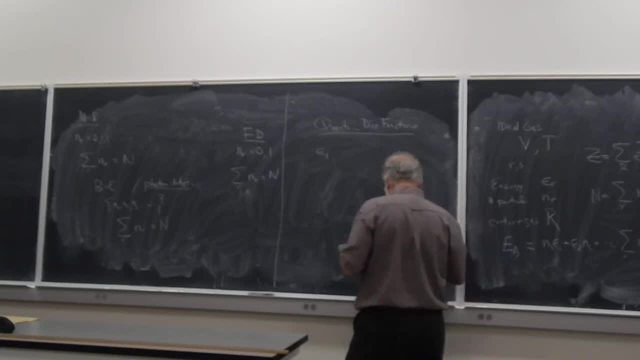 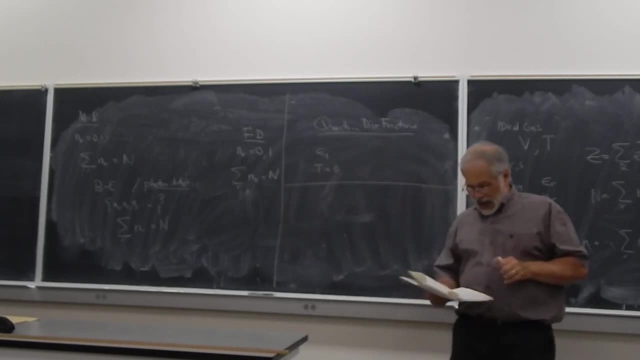 We said that it's in the ground state, then This, of course, is the situation at temperature equal to zero. On the other hand, with Fermi-Dirac statistics, I can't put more than one particle in that lowest energy state. 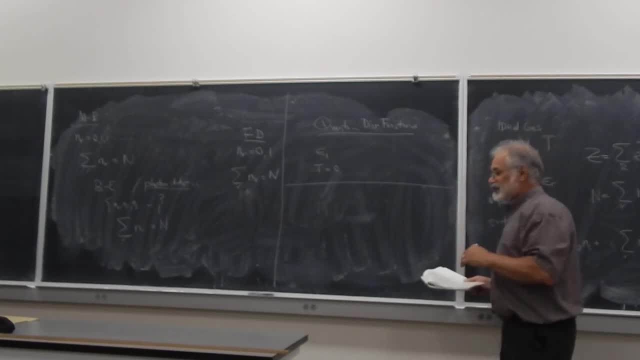 The states that I fill have to be of progressively higher energy until I've used up one particle per state. So the ground state configuration, so to speak, will look much different for a Fermi-Dirac or a fermion than it would for a boson. 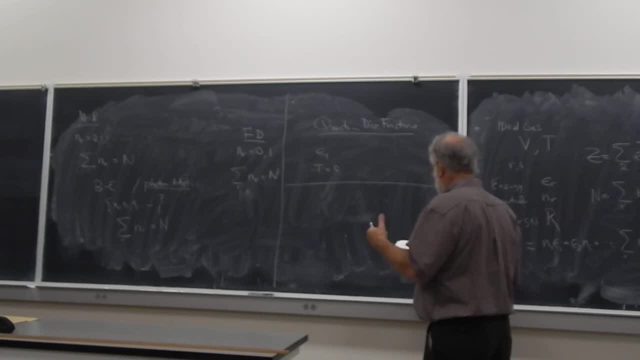 So we just have single particle states. all the way up. You can fill as many states as you have particles. Even at t equals zero, you're going to have particles that have a very high energy compared with E1, because we've got to fill progressively higher energy states. 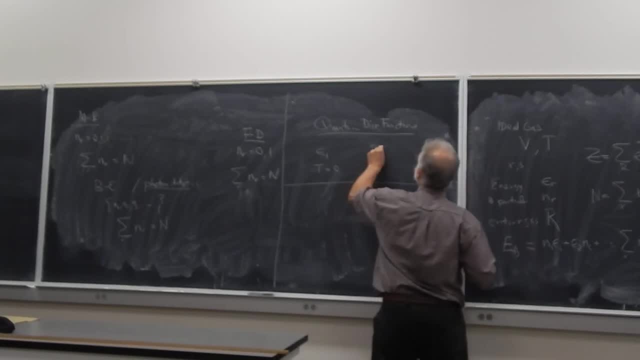 So in the Bose-Einstein case, the ground state energy is just going to be however many particles I have times E1.. In the Fermi-Dirac case, we expect that the energy of the ground state is going to be considerably greater than n times E1.. 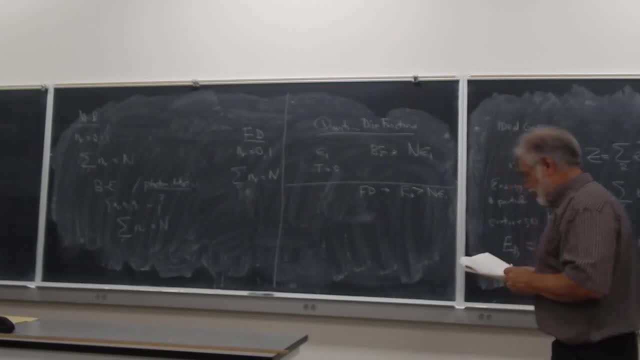 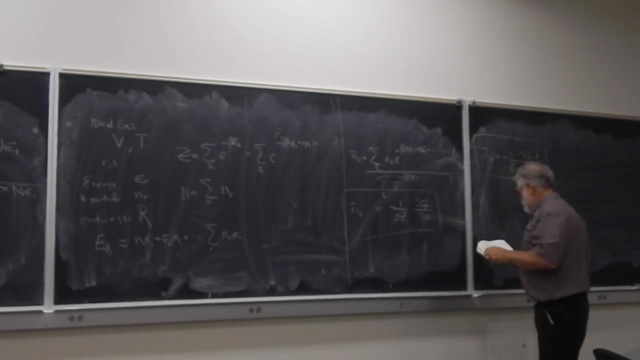 That's all because of the Pauli Exclusion Principle. Now I'm going to write down. in fact we did this before. if I want to calculate the mean number of particles in a state, I can write it in this manner: 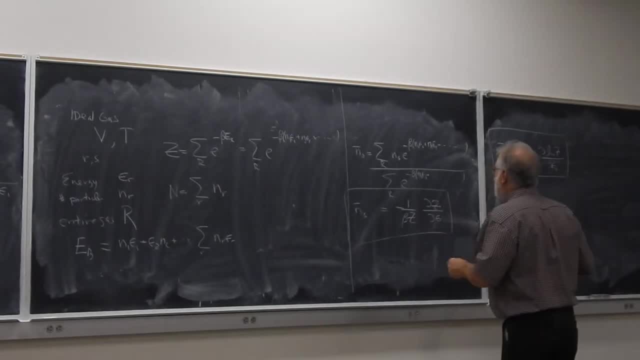 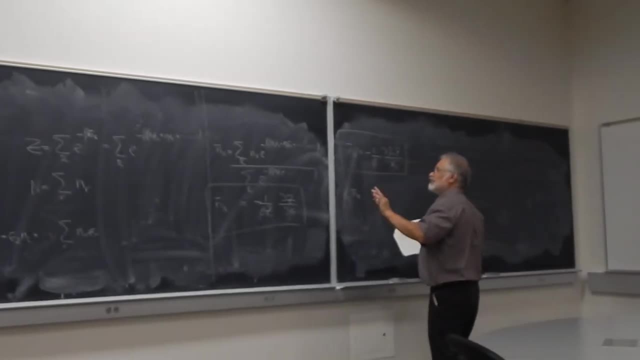 This will work for any of the distribution systems. but I'm going to play a little bit of a trick And I'm going to just factor out, in the case of the mean number of particles, and at n sub s, I'm going to factor out: 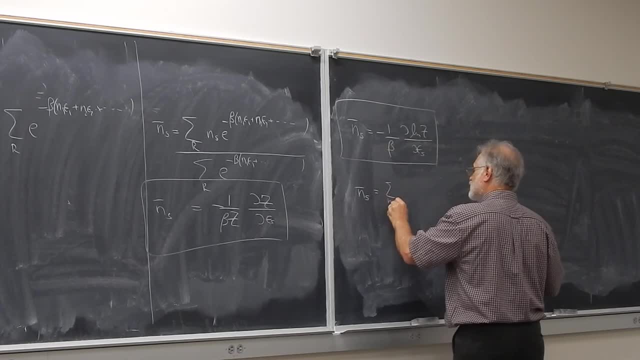 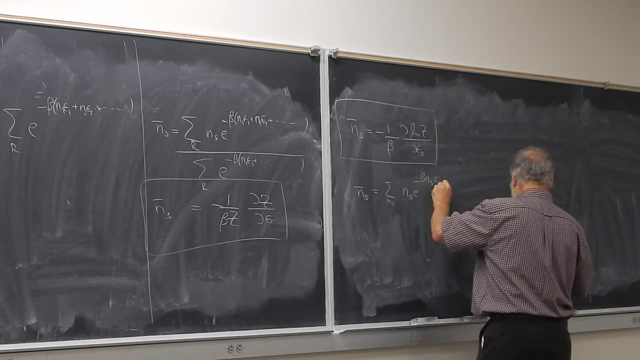 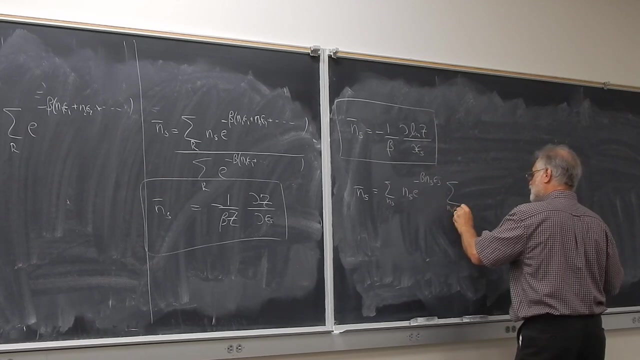 and I'm going to write it this way: the sum over n sub s times n sub s E to the minus beta, n sub s, E sub s times the sum over all the rest of the particles In the gas, n1,, n2,, everybody but n sub s. 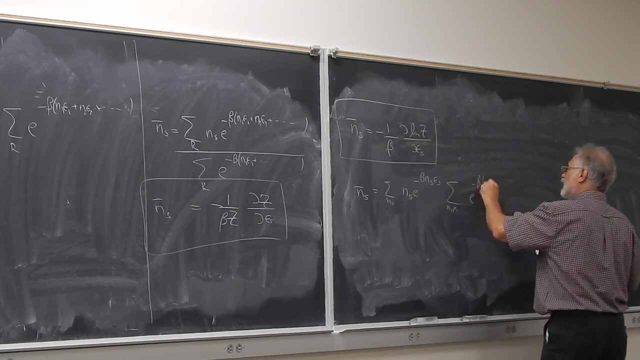 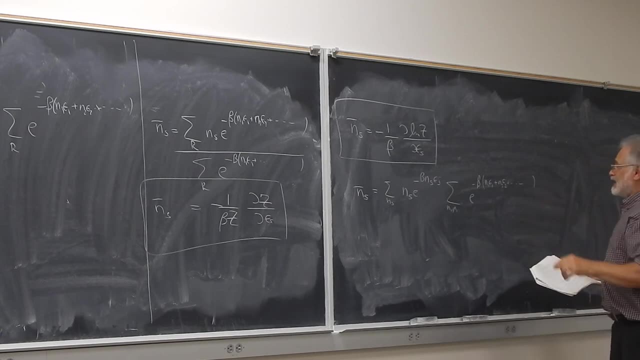 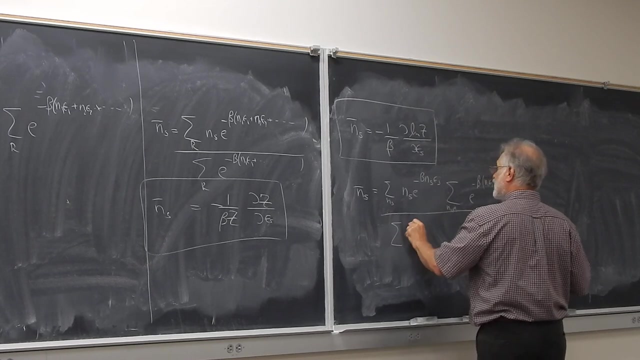 And here E to the minus beta: n1 epsilon 1 plus n2 epsilon 2.. That's all the way up, except for n sub s, E sub s. I'm going to divide that by E to the minus beta: n sub s, E sub s. 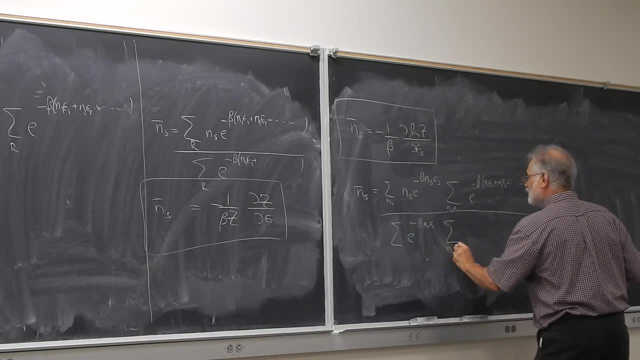 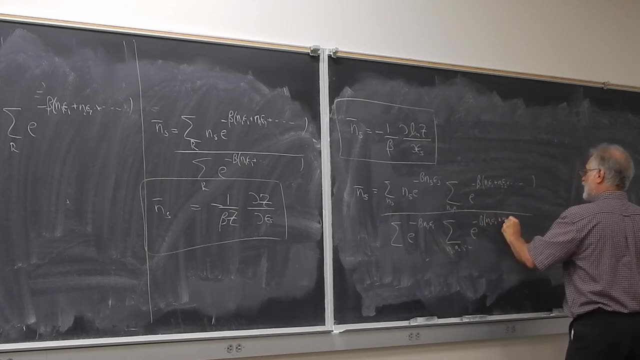 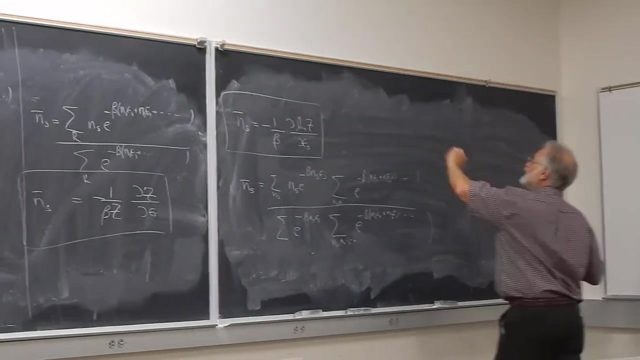 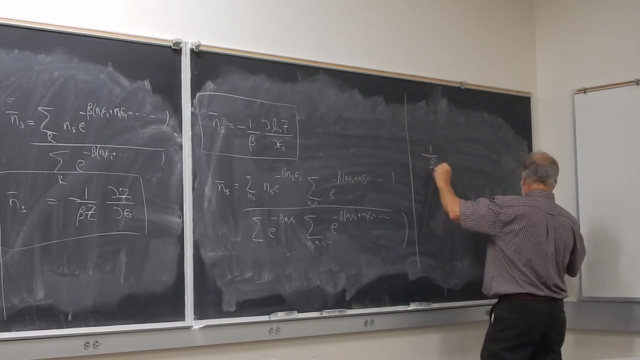 Again factoring the bottom and leaving this term the same, n2, et cetera, E to the minus beta: n1- epsilon 1, and 2- epsilon 2.. And notice immediately that I can write this: I can rewrite this expression as minus 1 over beta. 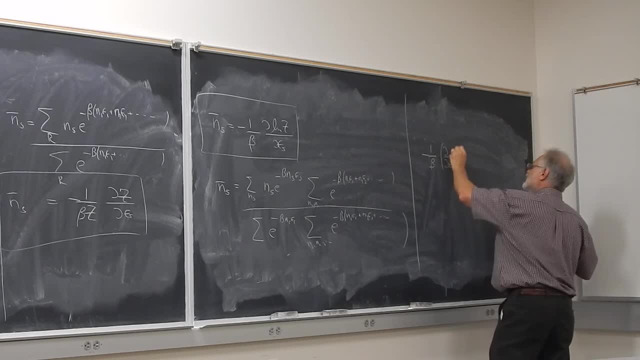 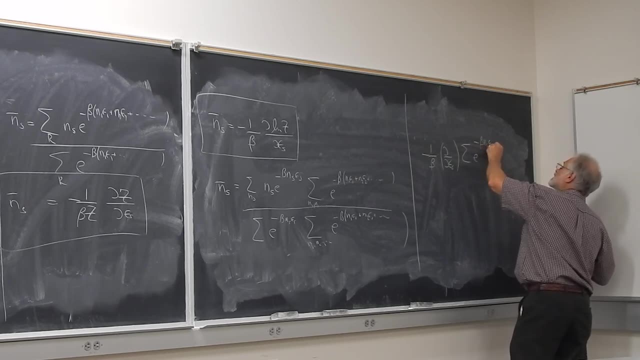 times d d E sub s of sum E to the minus beta n sub s E sub s Divided by sum E to the minus beta n sub s E sub s. Notice all summing over n sub s here. summing over n sub s here. 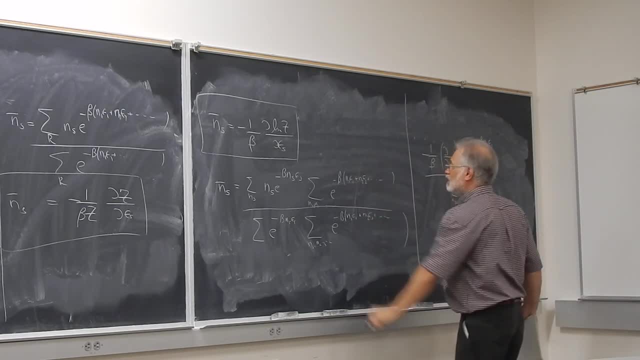 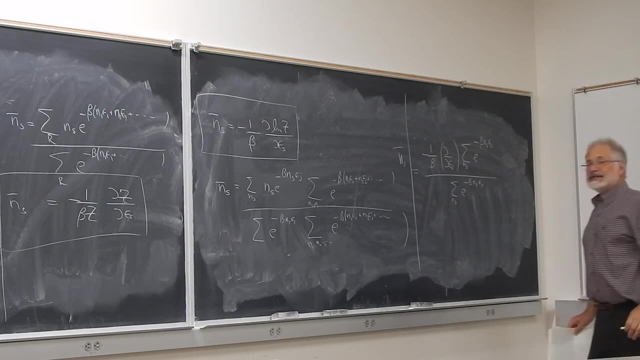 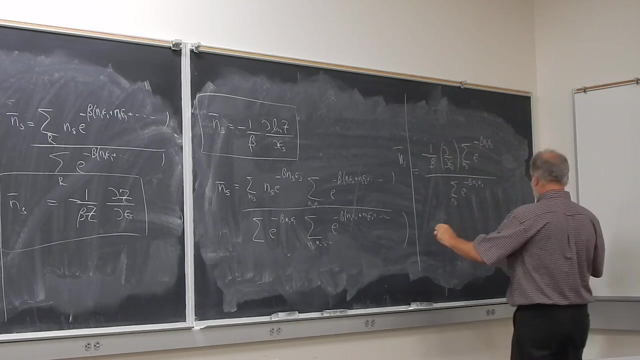 Notice these other guys have all canceled one another, So this is the mean number of particles I have at a state for n sub s. Now I can, I'll rewrite this in an even cleaner form. I'll write this as: n sub s is equal to minus 1 over beta d, d, E sub s. 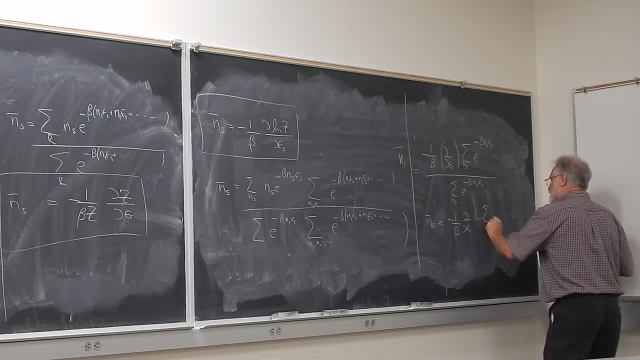 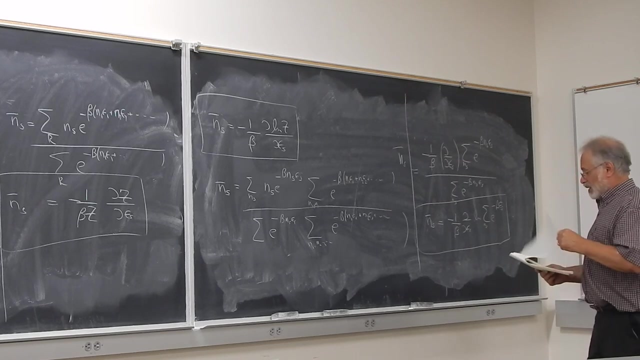 And that is a logarithmic curve: Log of sum n sub s E to the minus beta n sub s. This expression is valid for all three statistics, So it works in all cases. So, that being the case, let's take advantage of this expression and use it. 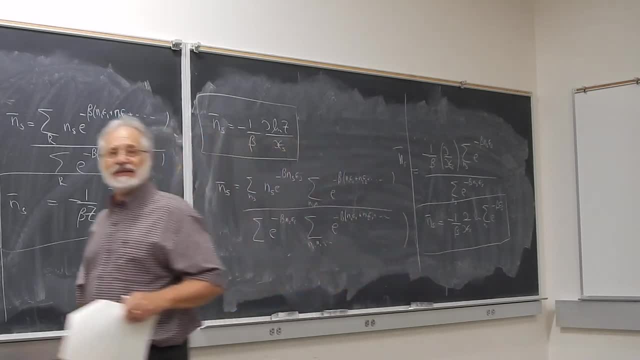 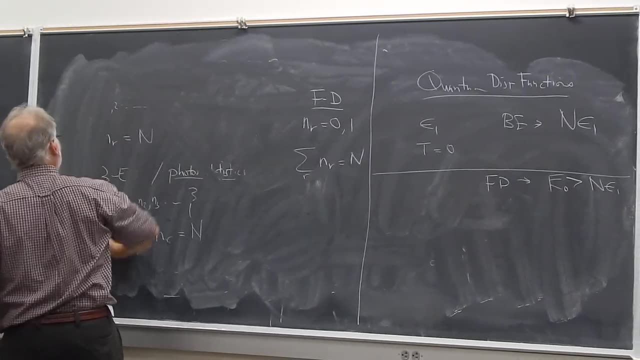 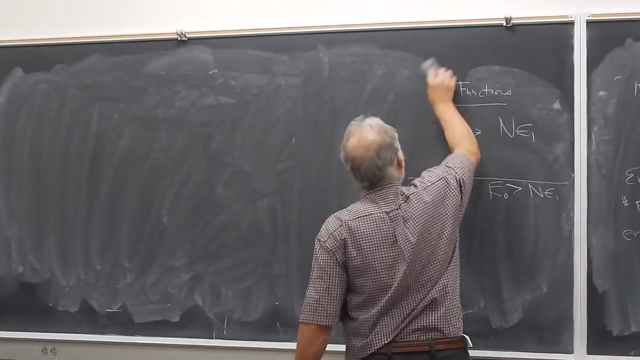 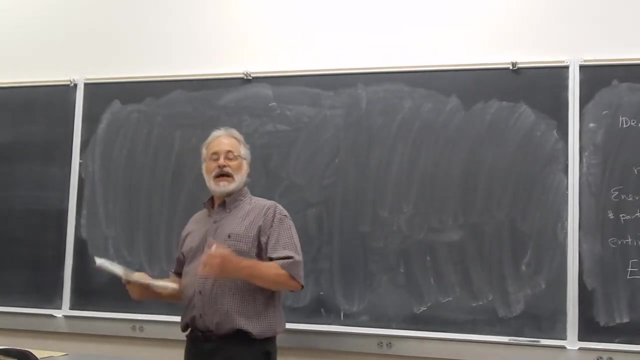 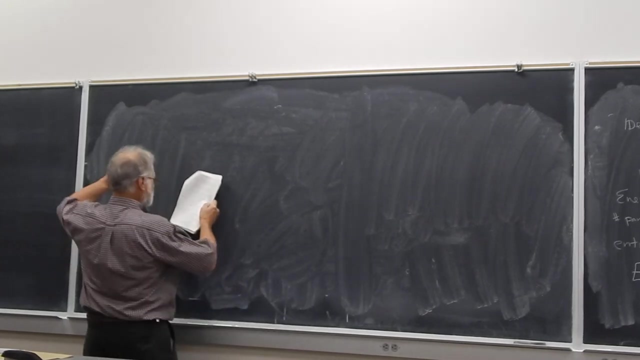 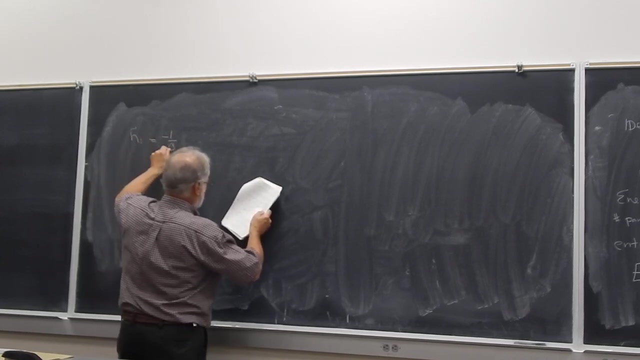 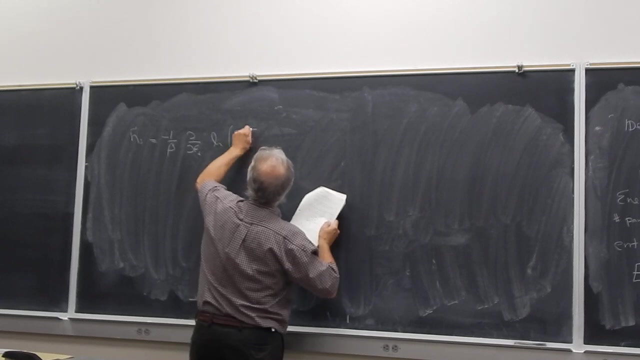 to examine the three possible cases of statistics. I'm going to start with the simplest possible case, Bose-Einstein statistics, but the photon statistics portion. This is really nice. I can write: n sub s is minus 1 over beta d d E s times the log of sum E to the minus beta E sub s. 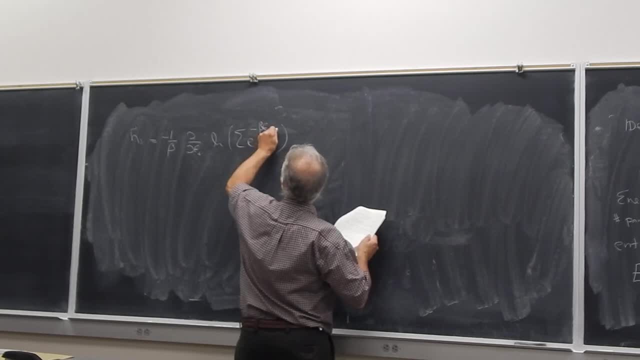 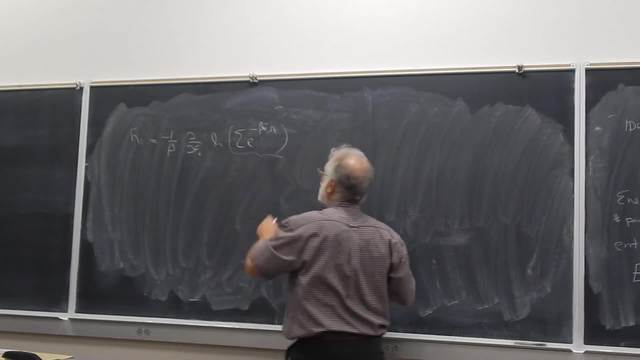 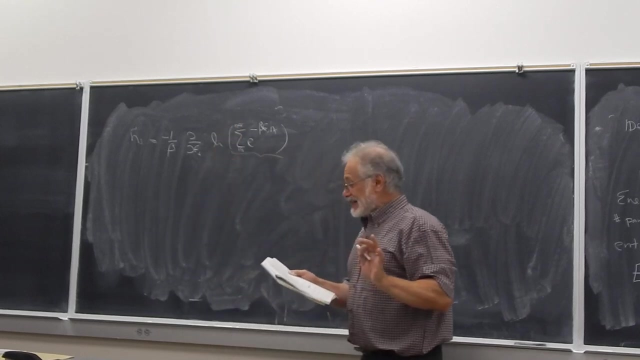 as I have before, Times n sub s. sorry, But I can sum this thing because it's an infinite sum. n, in this case, is not constrained. So this goes from: this is n sub s all the way to infinity. This is an easy thing to do. 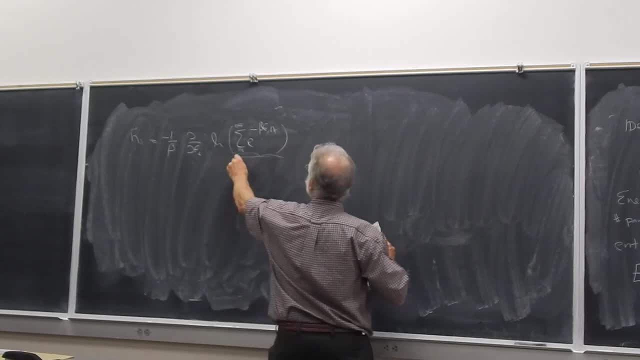 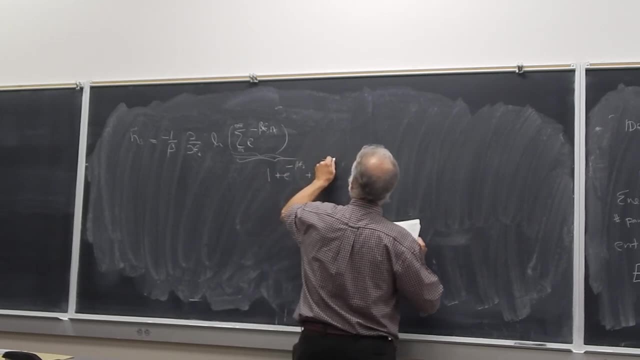 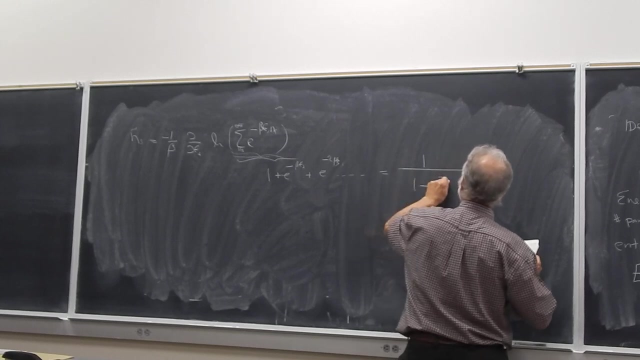 That sum, the sum of this series, I can write as 1 plus E to the minus beta E sub s, plus E to the minus 2 beta E sub s, And so on, And the sum of that series is well known. It's 1 over 1 minus E to the minus beta E sub s.